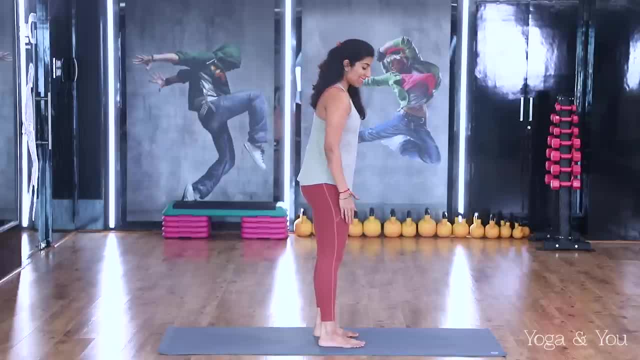 for you to get started. We are going to start standing with our feet wider than hip width and toes slightly turned out. We are preparing for Malasana. If you need a little bit of support for your heels, you can always roll up your mat or tuck a rolled up blanket. so 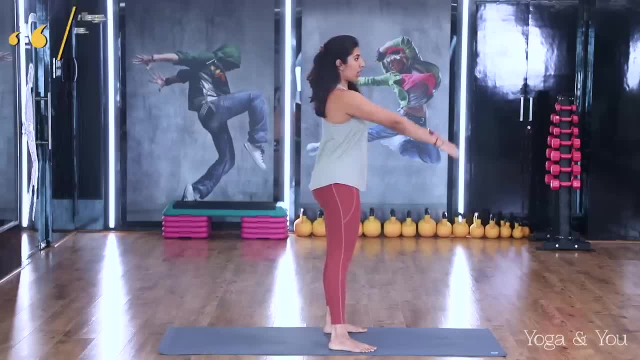 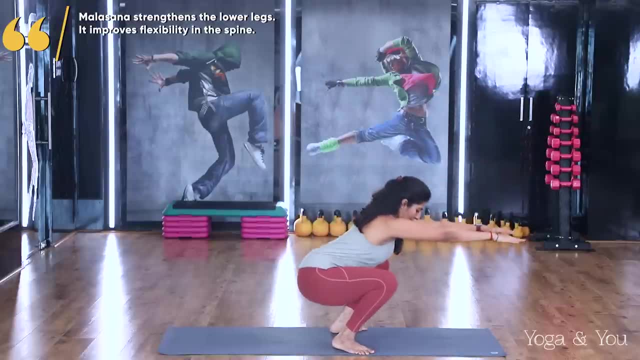 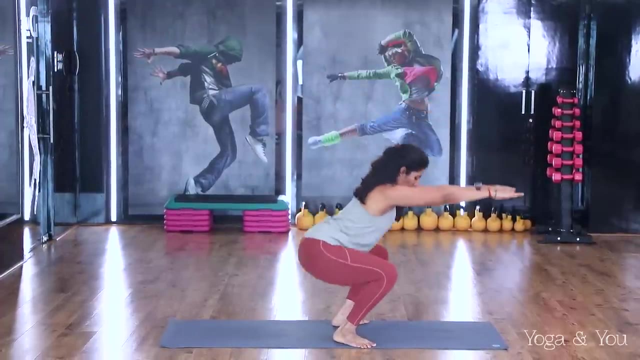 that your heels don't lift up As you inhale. you are going to take your arms up to shoulder level in front of you and as you exhale, just move your hips back. squat all the way down to the floor, Inhale and come back up. Fix your gaze at one point, Exhale and squat. 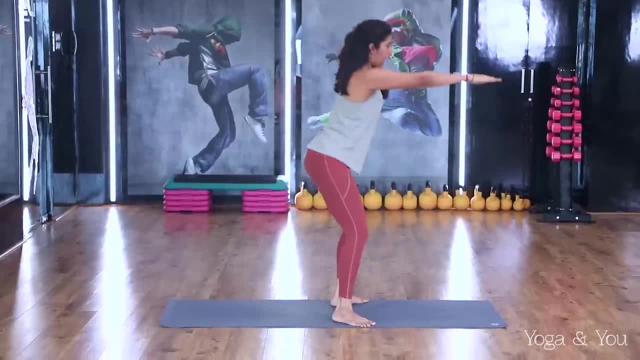 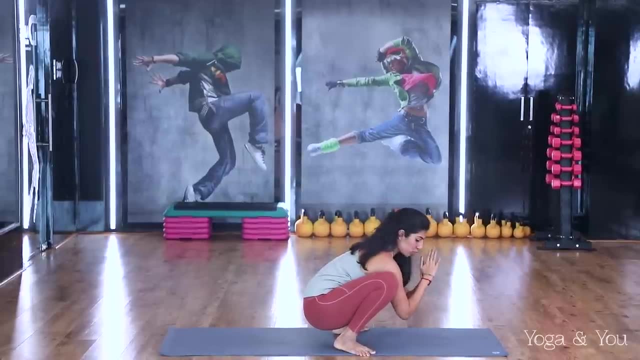 all the way down. We will do this one more time: Inhale and up, Exhale, squat all the way down. This time you bring your palms to the heart centre, Namaste, Use your elbows to push the knees open, Send the chest up and let's hold it here for three. 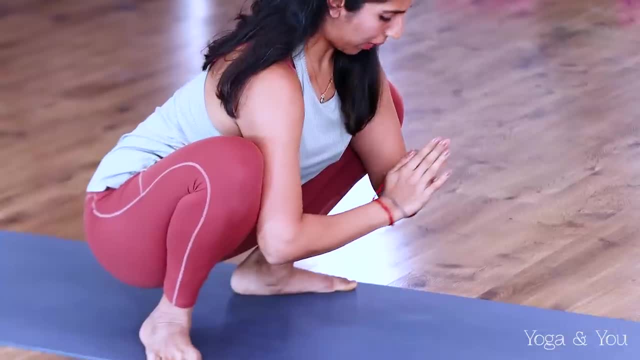 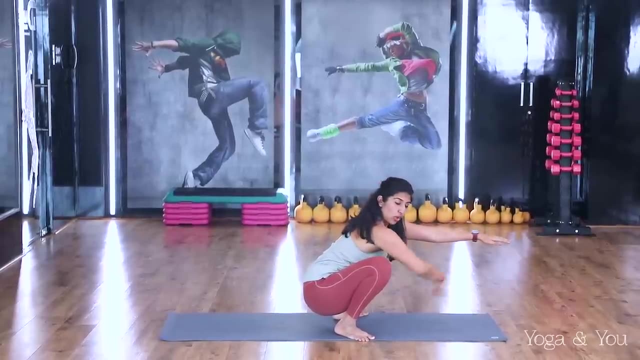 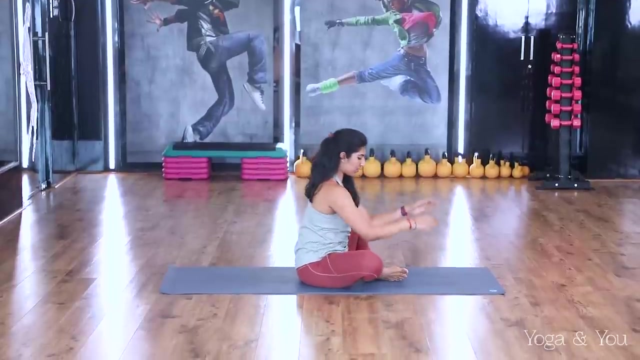 Two And one. Let your hips open up nicely. Now stretch your arms forward, keeping the knees nice and wide, With control. draw your lower belly in and very slowly release your hips to the floor and you are going to bring your feet together. soles of the feet touching. 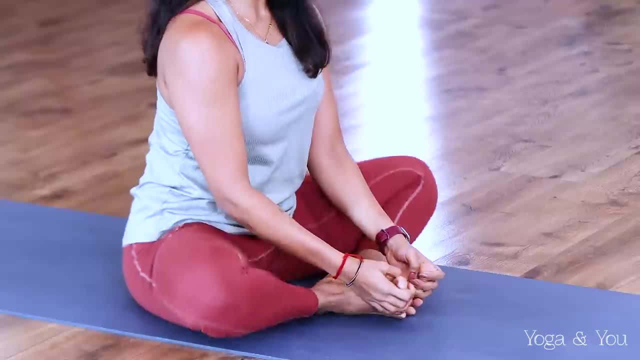 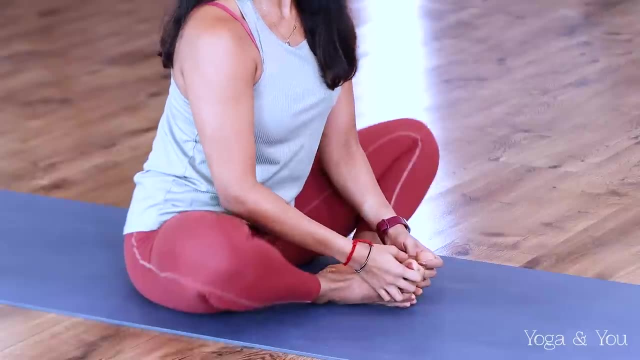 each other in Baddha Konasana. We are just going to open up a little bit by flapping the knees up and down a few times. Find a little release in your inner thighs, Then we are going to do a little bit more. 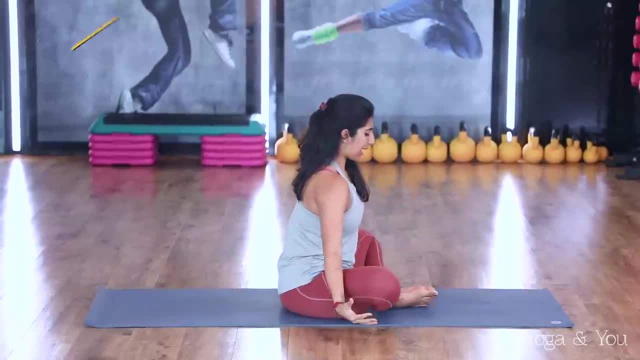 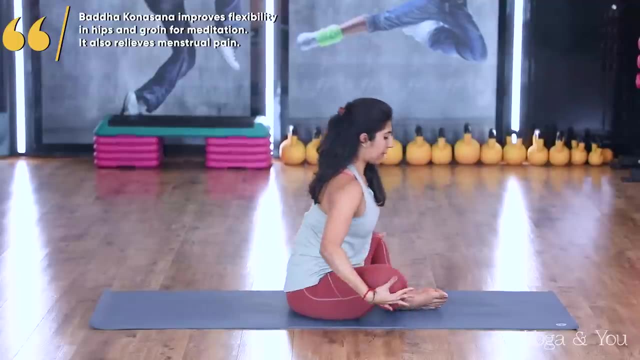 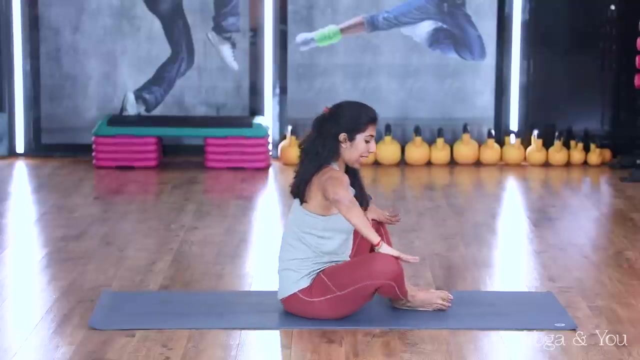 Active opening using your palms. So as you exhale you bring your knees in together. Inhale: you are going to use your palms to move the knees out, lean forward slightly. Exhale, Inhale, Exhale, Inhale. Be gentle with the push, don't overdo it. Exhale, Inhale. 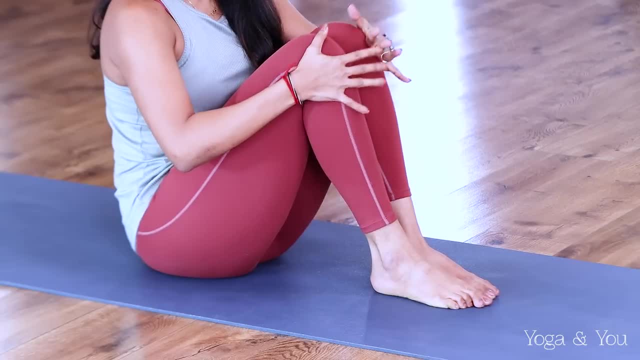 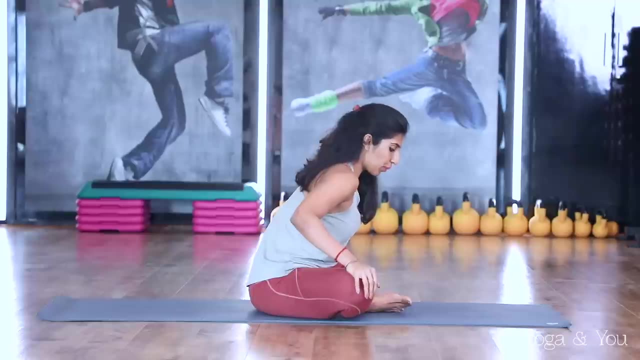 At every point of the practice, you keep listening to the body, listen to your breath and you will know how much you can go. One more time, Inhale, Last one And inhale. You are going to start to open out the legs. Mat width a. 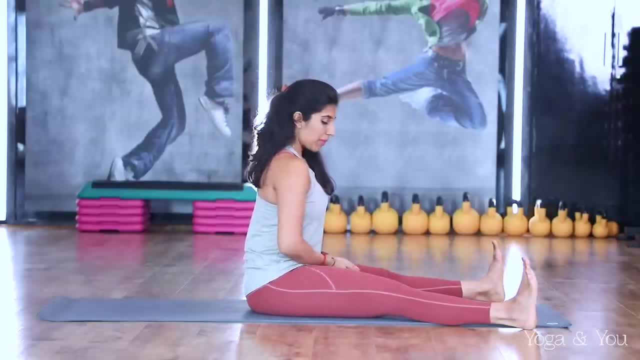 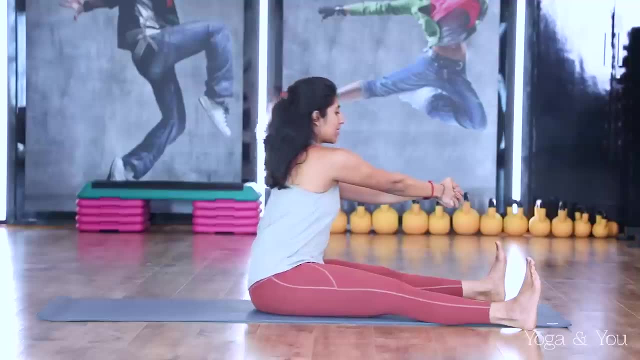 little wider than that. Your toes are up. Send the heel forward, Make space between the thighs, Keep the spine tall, Your belly engaged, Interlock the fingers. We are going to start to make big circles reaching towards your toes with the spine lengthened. So if 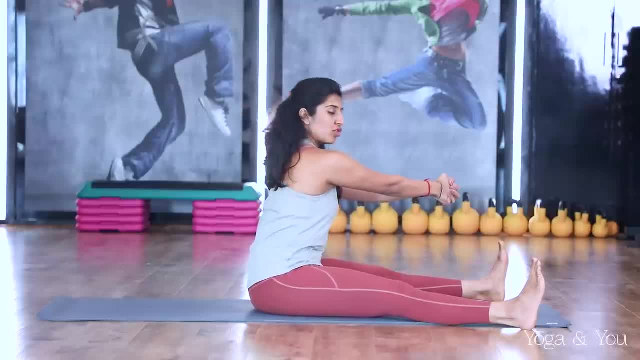 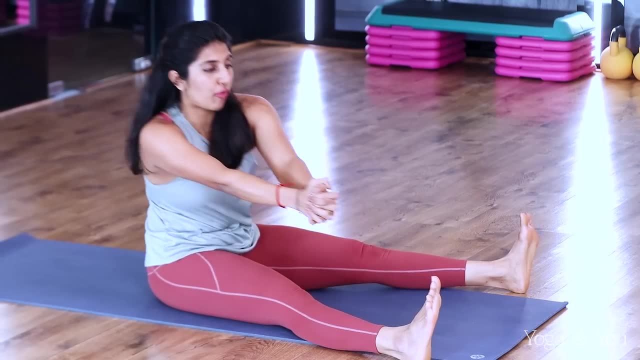 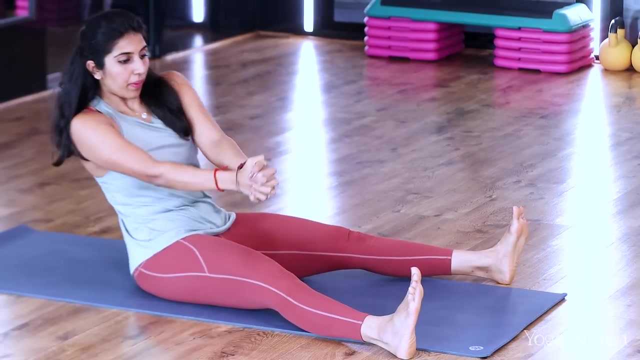 you are not able to go beyond this. don't start to round your back. Stop here: Two, Three, Four And four, Coming back to center, and let's switch to the other side: One, Two, Three And four. 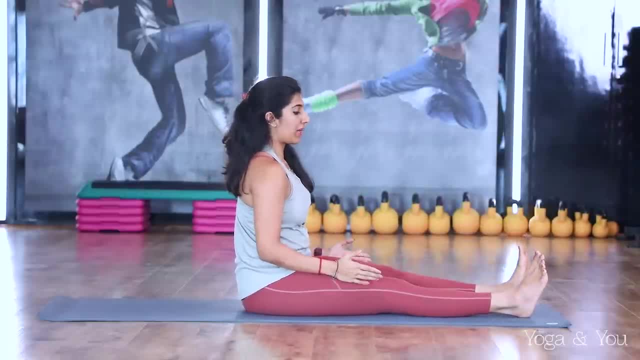 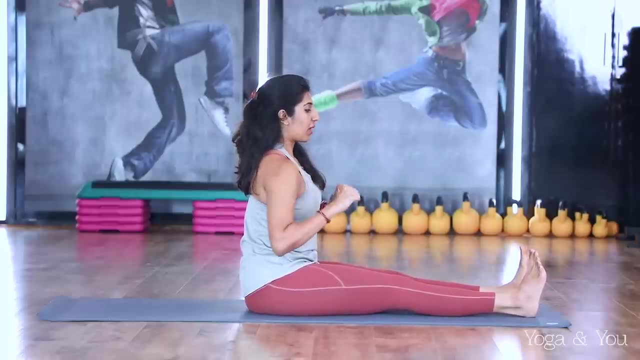 Back to center, Bring your feet a little closer to each other. It doesn't have to be touching Parallel. You are going to grip your fist this way, Like you are holding an oar, Like you are rowing a boat. Okay, So you are going to go forward and lean back One Forward. 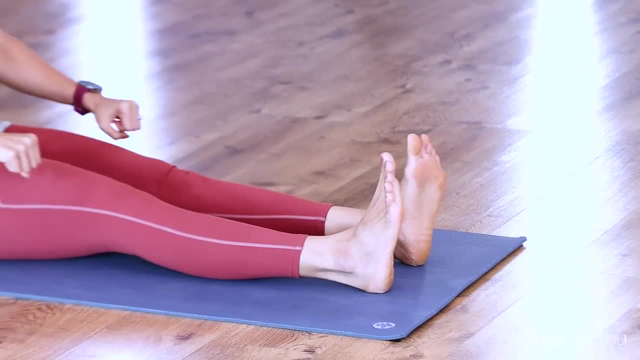 Engage your belly when you are moving back: Two, Three, Four And four. Coming back to center: One, Two, Three, Four And four. Moving back: Two Forward And back, Three Forward And back, Four Forward Back, Five. One more Forward And back. Just for a moment. 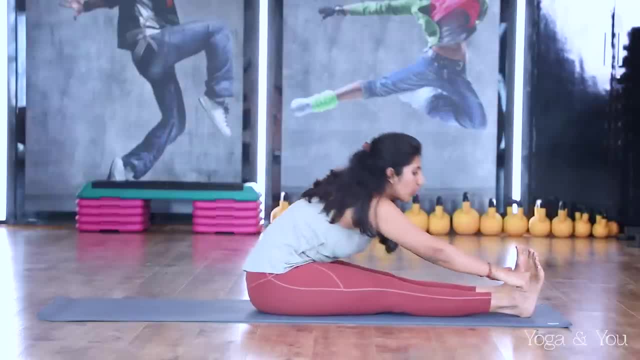 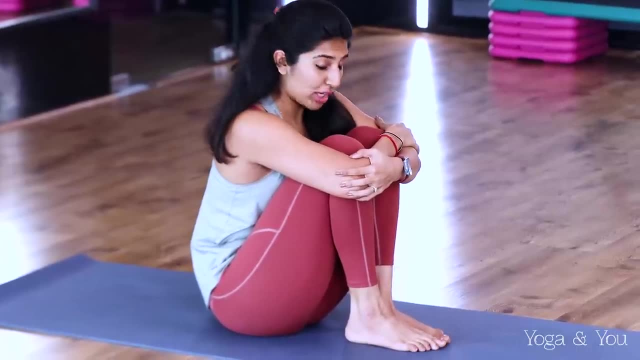 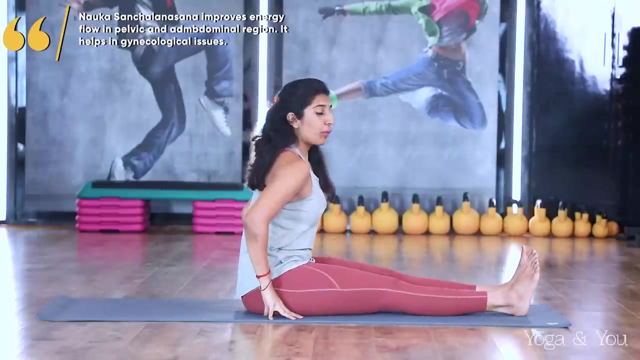 bend the knees. That was Navaka Sanchalanasana. Like you are rowing a boat As you inhale. you are going to relax Now you are going to bend your right knee and bring the heel in towards the groin Inhale. 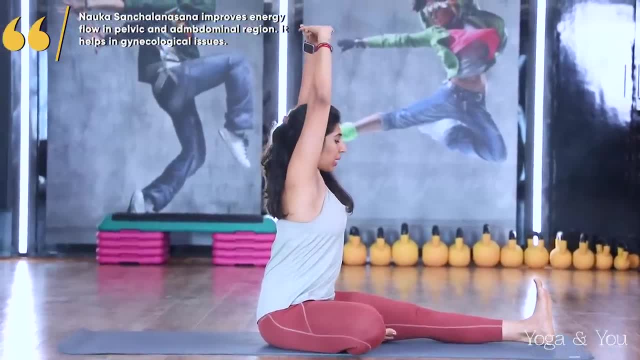 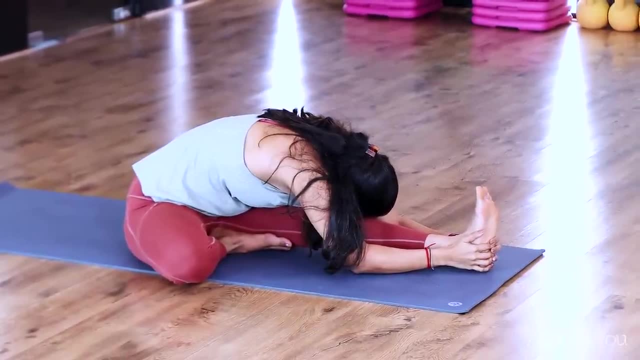 Inhale, Lift your arms up, Interlock the fingers. Stretch up Toes flexed. Exhale. Fold forward into Janu Sirsasana. Hold it for a breath. Next inhale, Interlock And. 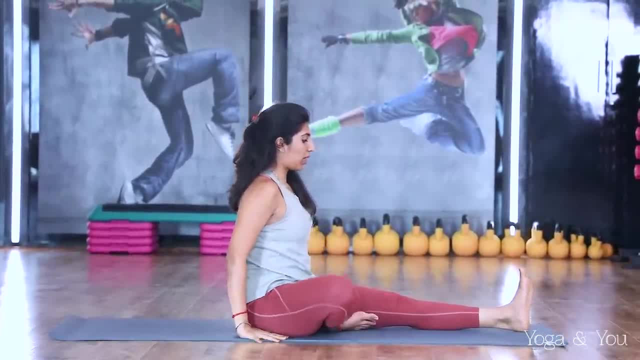 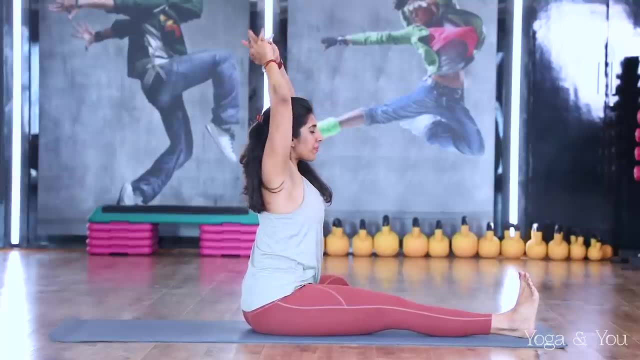 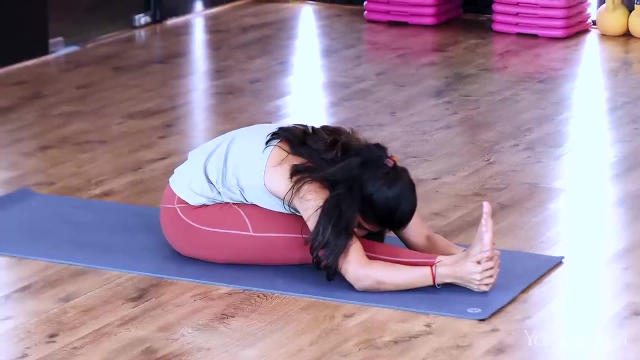 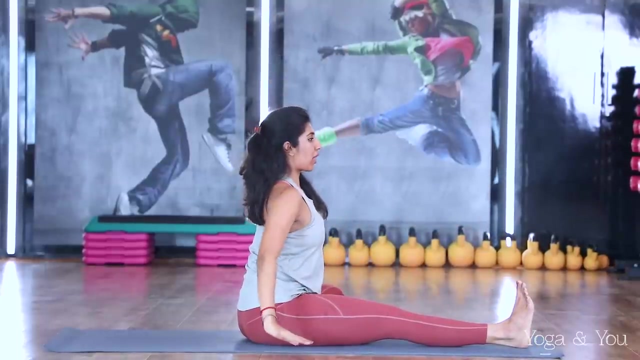 come up, Exhale, Bring your arms down. Switch sides: Right leg forward, Left heel towards the groin. Inhale Arms up, Exhale And fold forward. Stay for a breath, Inhale, Interlock the fingers. Inhale Up, Exhale, Bring your arms down. Now you are. 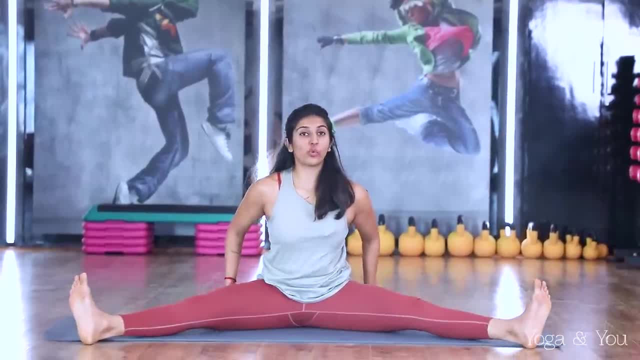 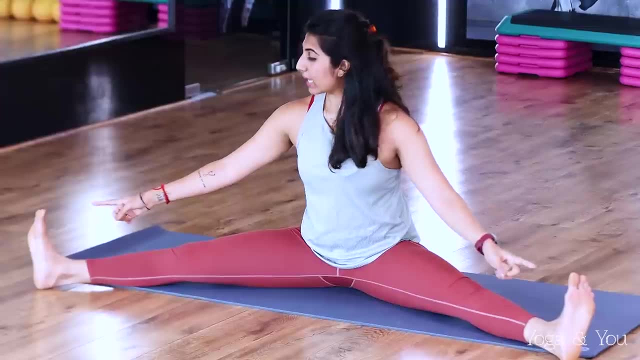 going to open out the legs, nice and wide, As wide as you can go. You can even use your palms to slightly move your hip forward. You find that opening in your inner thigh. Keep the toes pointing up, Palms in front of you, Inhale As you exhale, step forward, Stay. 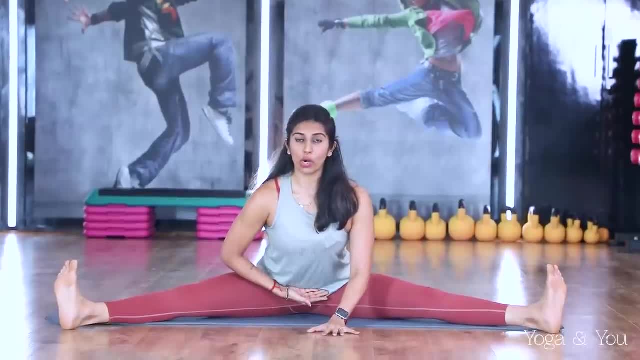 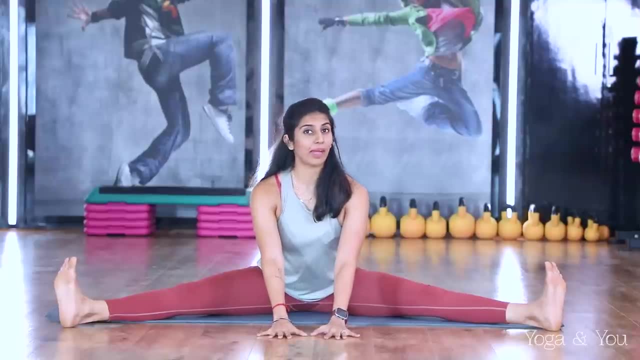 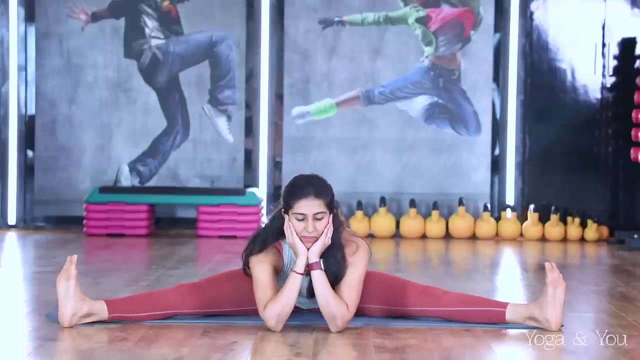 still Step forward slightly. You are lengthening from the lower back. Inhale again, Exhale Little bit. more. Inhale Last time. if you can place your forearms down, You can even cup your cheeks with your palms And you are going to stay here. Let the inner thighs open. 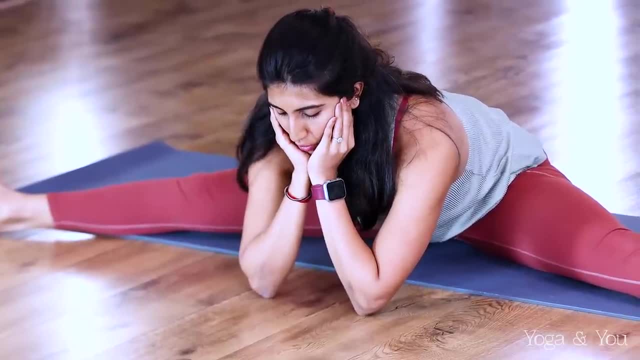 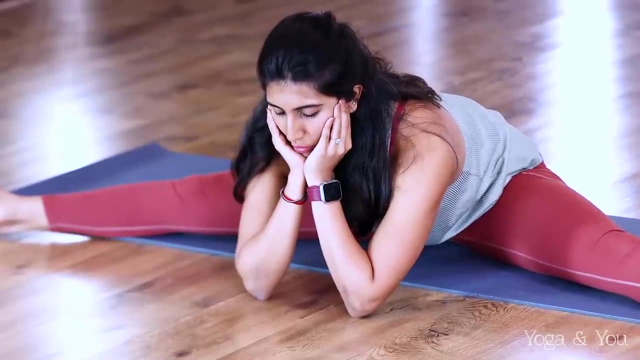 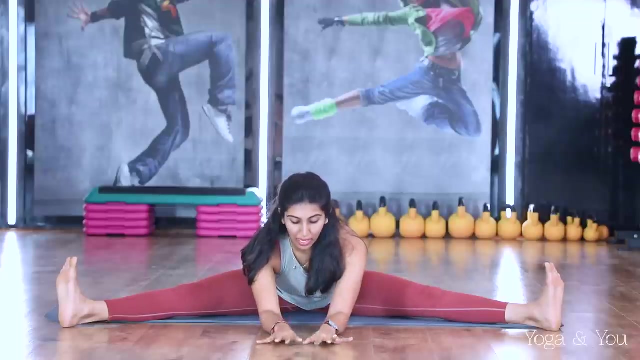 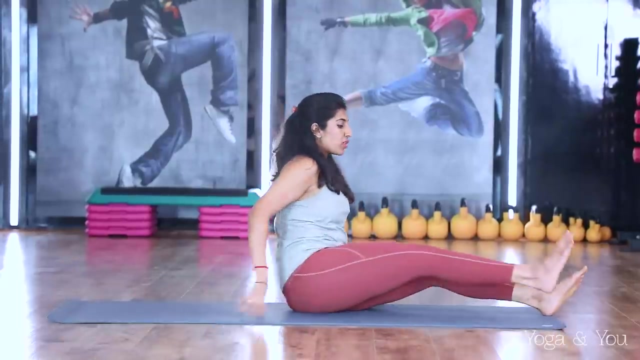 up. Keep your face relaxed, Lengthen from the lower back. Let's take two more breaths. Just enjoy that opening One more. Slowly release your palms And you are going to walk your palms back. Coming back to the top of the mat, let's prepare for Paschimottanasana. 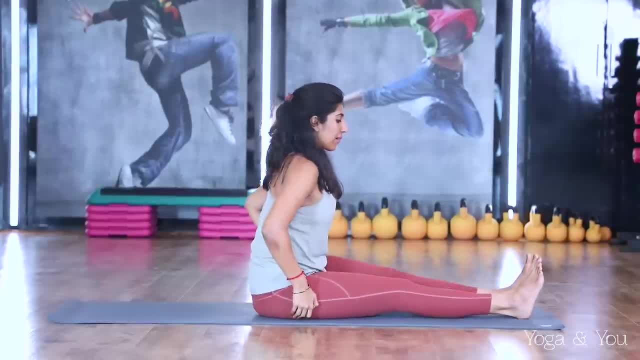 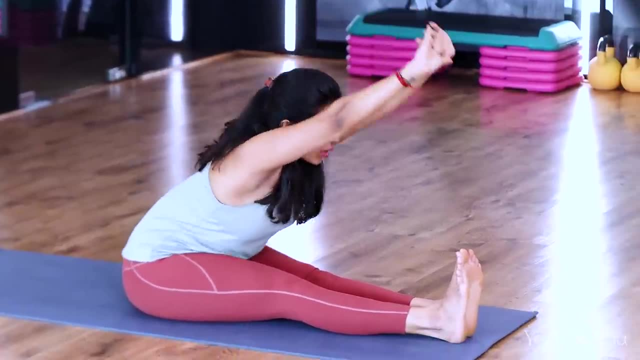 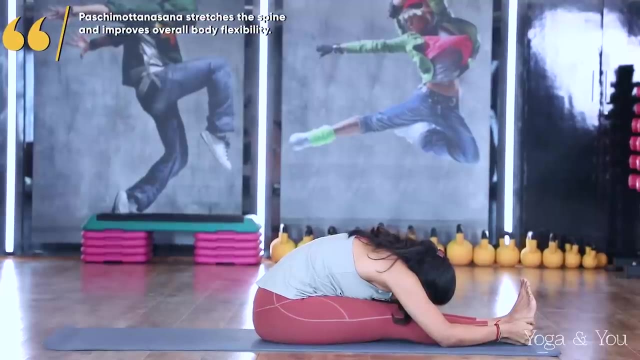 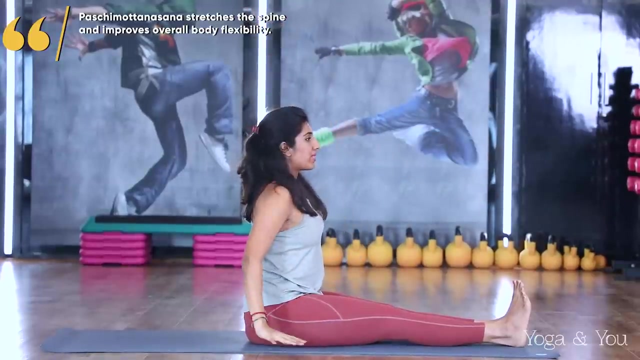 You start in Dandasana, You release the hips a bit. Toes up, Inhale, Arms up, Exhale. Lengthen forward from the lower back, Go all the way down, Interlace the fingers, Inhale Up, Exhale. Bring your arms down Now, if Paschimottanasana. 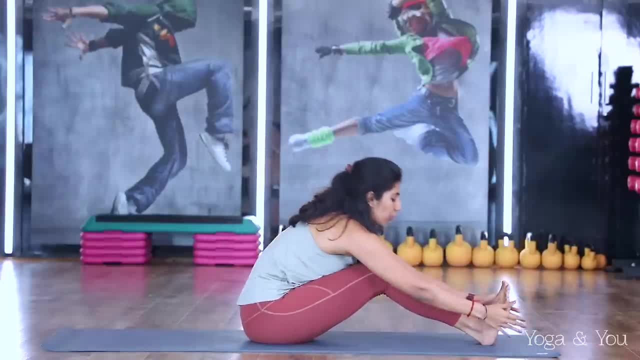 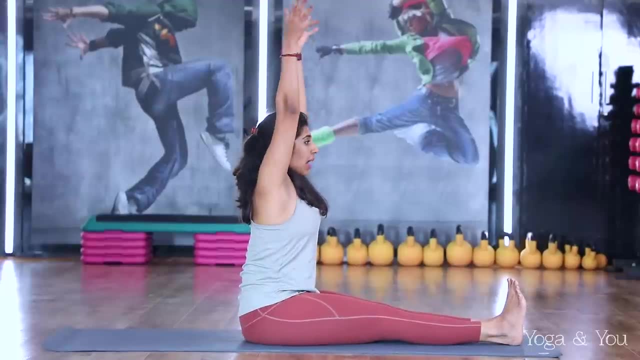 is difficult for you. you can always bend the knees and fold forward, or use a strap to get into the pose. We are going to practice one more time: Inhale Arms up. Choose the modification that is most comfortable for you. Exhale- Fold forward. Inhale Arms up. 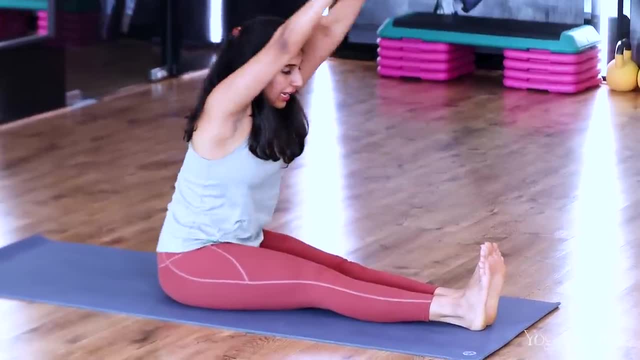 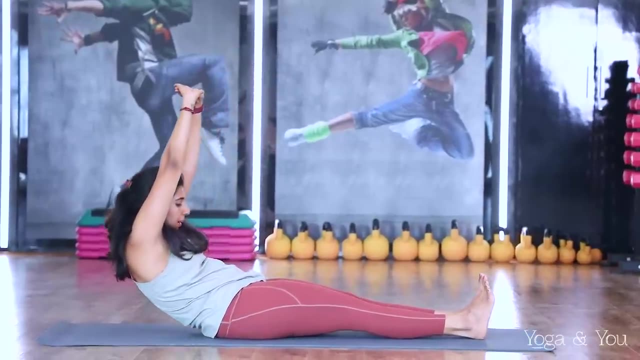 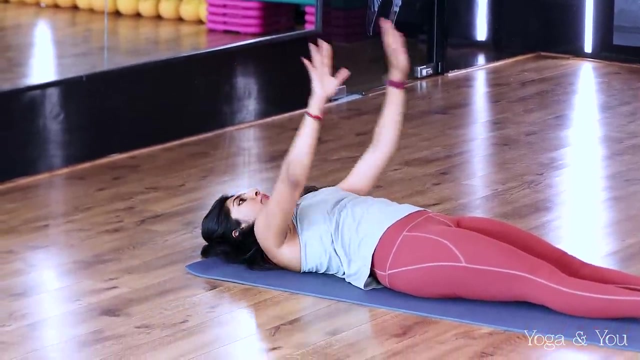 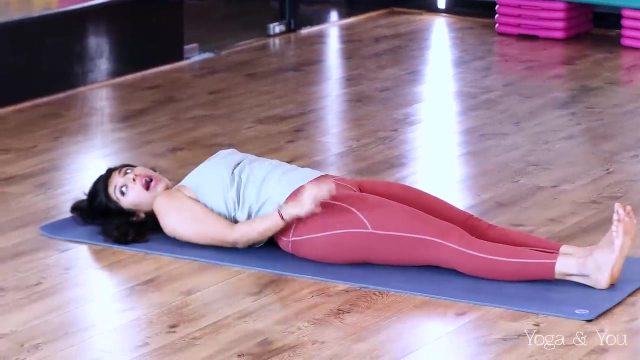 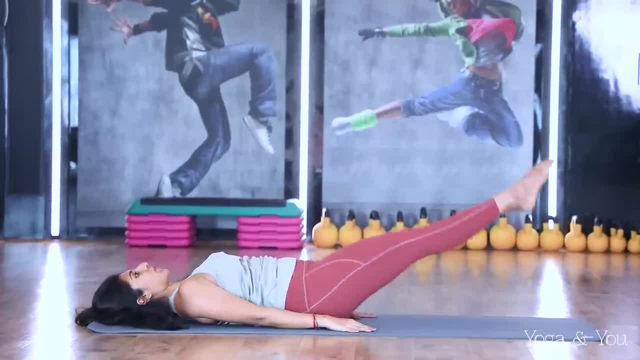 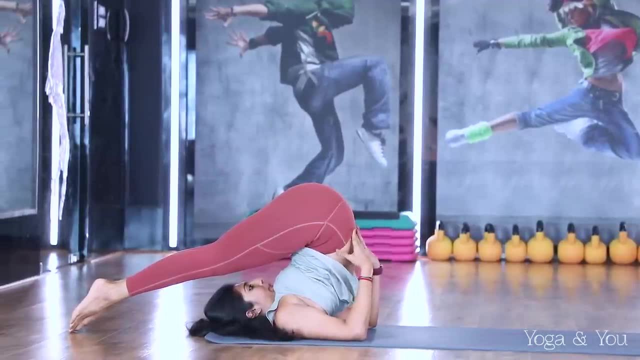 We are going to go up directly into Halasana. As you exhale, lift the legs straight up using using your belly. lift the hips up, take the feet behind you, support your lower back with your palms, adjust the elbows, release the feet to the floor. breathe here. 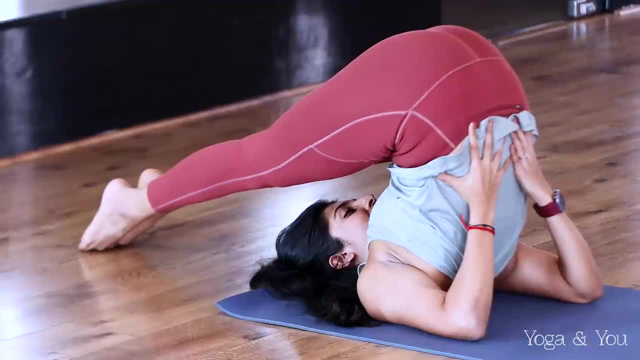 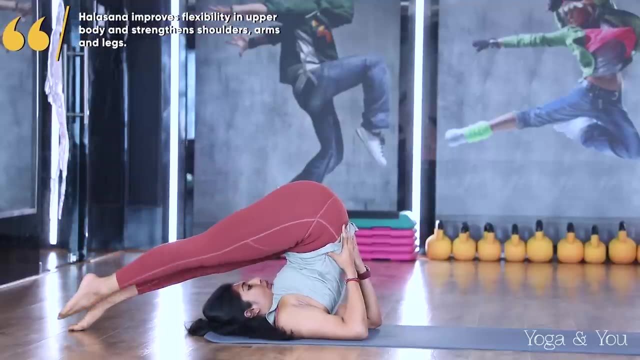 if you're on your period, avoid inversions. you can also use a wall, or you can use a chair behind you to rest the feet, so you don't have to go all the way down to the floor. choose the modification that suits you best. on your next inhale, start to roll down vertebra. 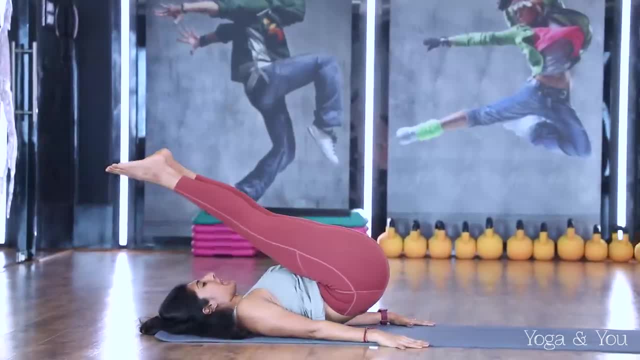 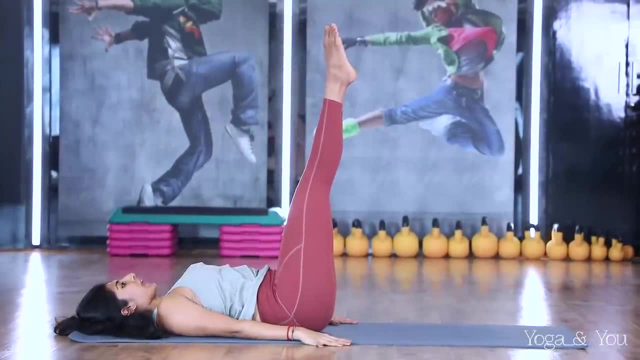 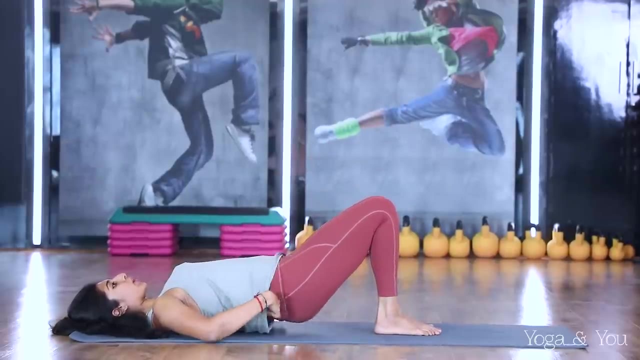 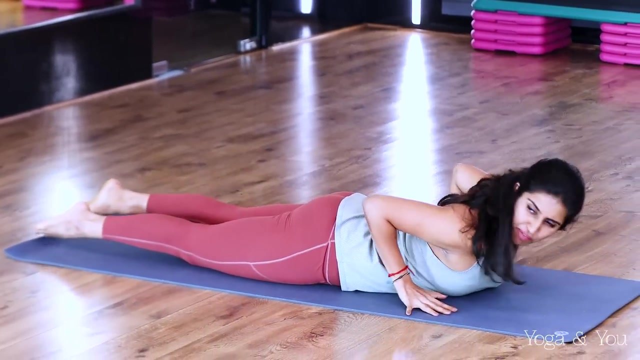 by vertebra. find control from the lower belly so you're not releasing with a jerk, it's a very controlled release. after you get to 90 degrees, you can bend the knees and slowly place your feet down for the counter pose. we're going to do Bhajasana, so you can turn around, lie down on your belly, keep the feet slightly apart. palms: 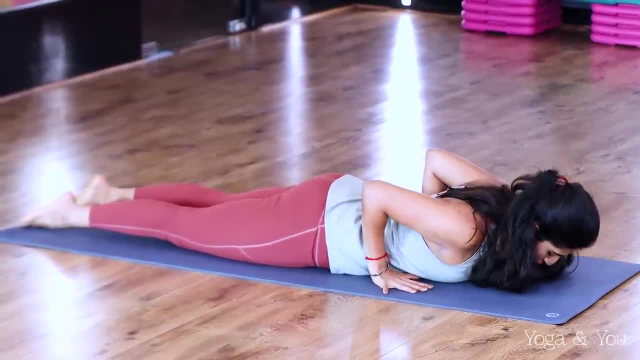 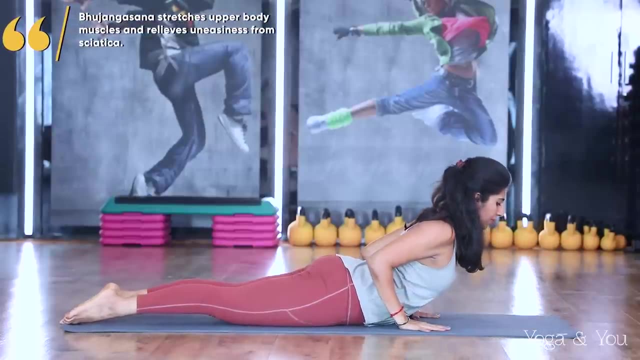 next to your ribs, a little lower than the chest, forehead to the floor. inhale elbows in towards the body, lift up, exhale down, inhale up, exhale down. we're gonna do it one more time. maybe. if you have any questions, you can ask us, or we can be happy to answer them in the next video. 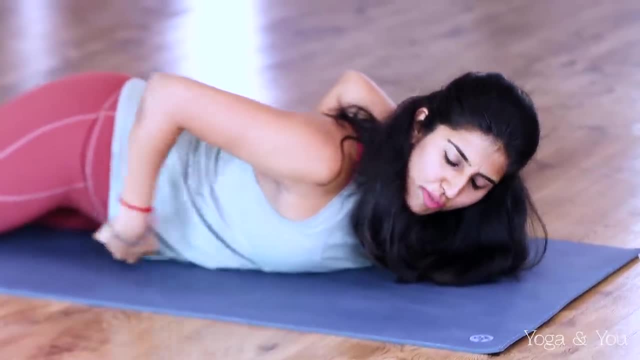 or if you have any questions, we can answer them in the next video. if you have any questions, you can ask us or we can be happy to answer them in the next video. Make sure the lower belly is still rested on the floor. Little bit of pressure there. 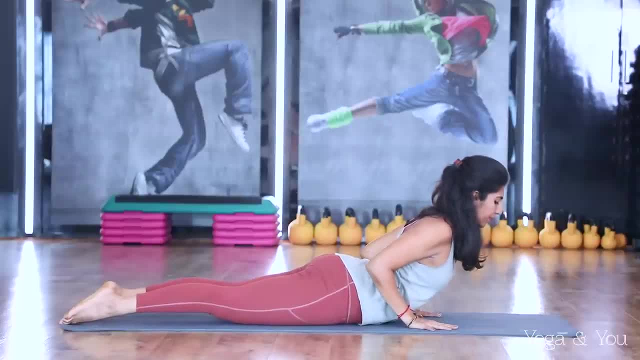 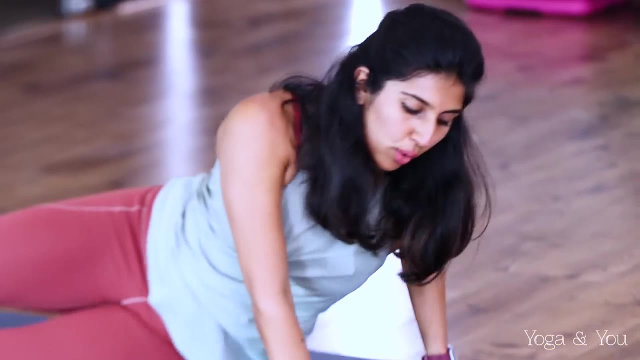 Inhale, lift up, stay 1,, 2,, 3,, 4,, 5.. Exhale all the way down, Turning around again, lying down on your back. You're going to hug both knees into the chest. 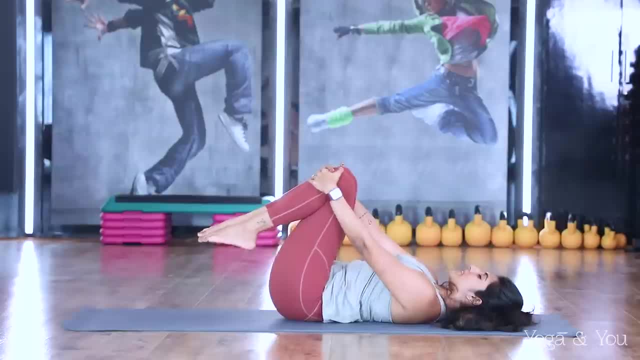 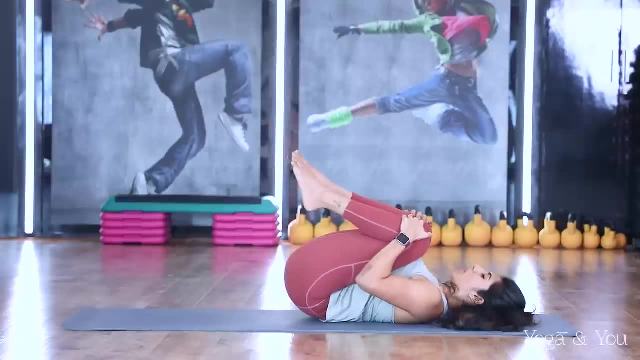 Upana Asana. dynamic Inhale release- Exhale hug. Inhale release- Exhale hug. One more Inhale release: Exhale. bring the knees in close. 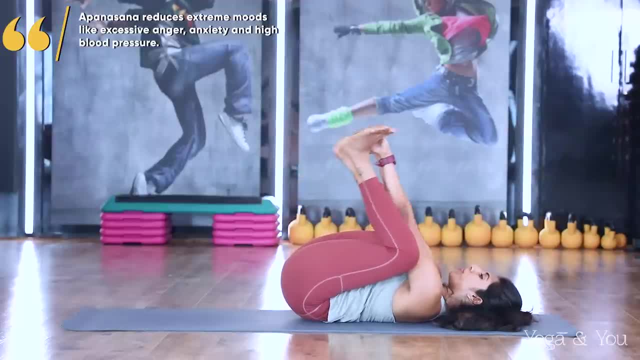 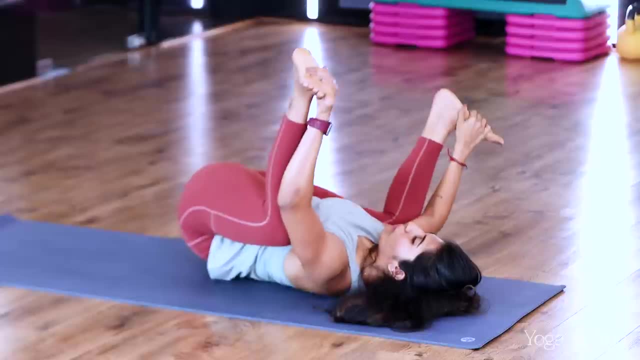 Take your arms in between your legs. Hold on to the arches of your feet, Moving into happy baby. Open out the inner thighs, Get the knees closer and closer to the floor, If your body allows. gently rock side to side. Inhale about three times on each side.